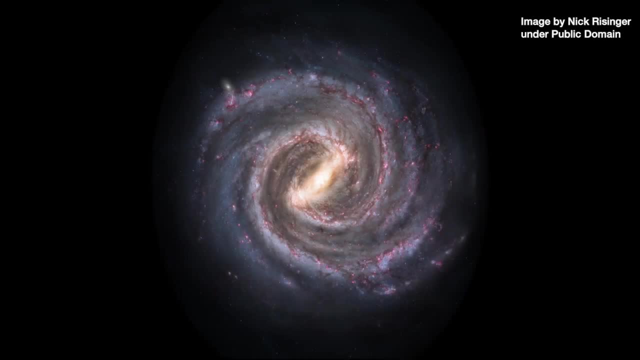 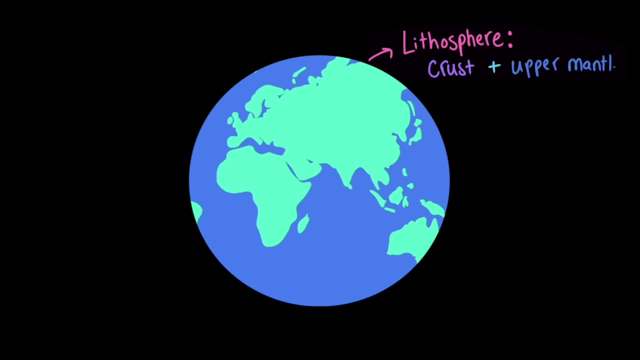 the Milky Way galaxy. But there's another kind of movement that happens slowly in the rock beneath your feet. Earth's lithosphere, which is made up of the crust and the upper part of the mantle, is broken up into pieces called tectonic plates. These plates move around on top of the asthenosphere. 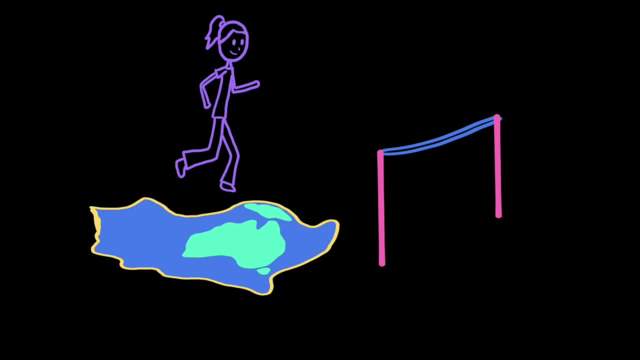 which is the section of the mantle just below the lithosphere. Don't bother racing a tectonic plate, because your victory would be guaranteed. Tectonic plates typically only move a few centimeters in a year, which is about as fast as your fingernails grow. However, after millions of years, those 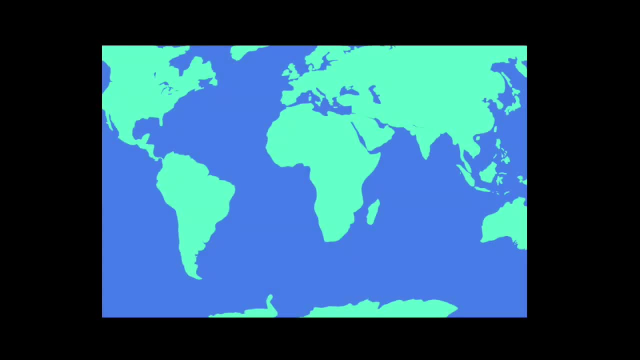 distances add up. This means that the Earth hasn't always looked the way it does now. Scientists believe that the Earth is moving around on top of the asthenosphere, which is the section of the Milky Way galaxy. So if we can just imagine the Earth moving around on top of the asthenosphere, 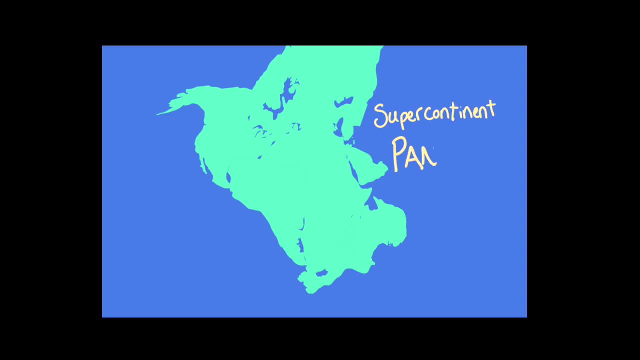 we can imagine the Earth moving around on top of the asthenosphere, which is the section of the Milky Way galaxy. So imagine if the continents were once all connected in one big supercontinent called Pangea. Just imagine if the continents were still connected today. You could drive from. 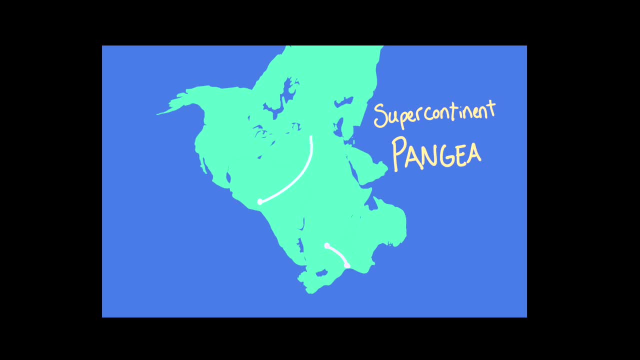 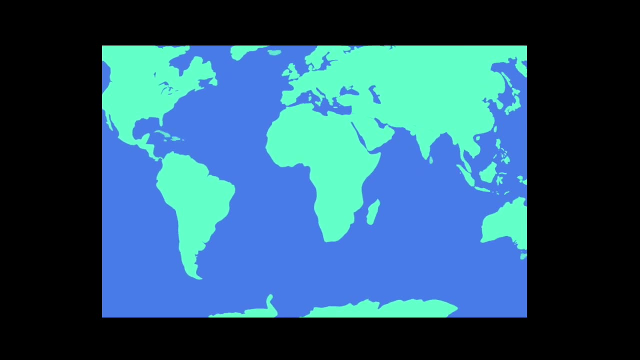 Africa to Antarctica, or even take a train from South America to Europe. Over 200 million years Pangea broke apart and the pieces drifted into the continents we know today. So if the plates move so slowly, how do we know that they move at all? Scientists have documented evidence from 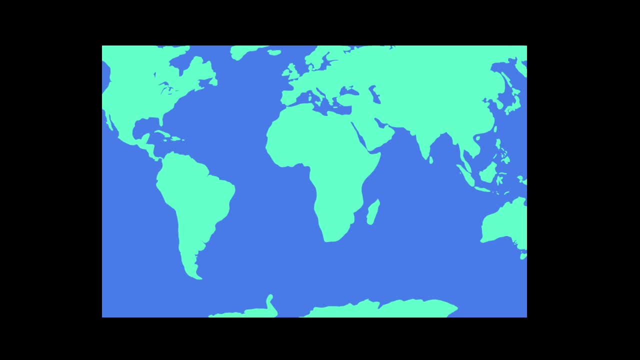 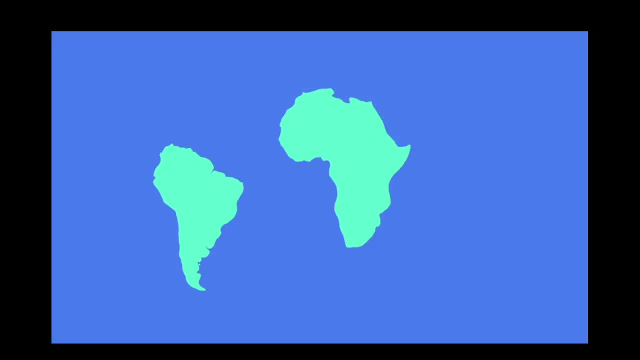 various features on Earth that support the theory. So if the plates move so slowly, how do we know of plate tectonics? If you cut out the continents on a map, you can see that they almost fit together like a jigsaw puzzle. For example, the east coast of South America looks like it could. 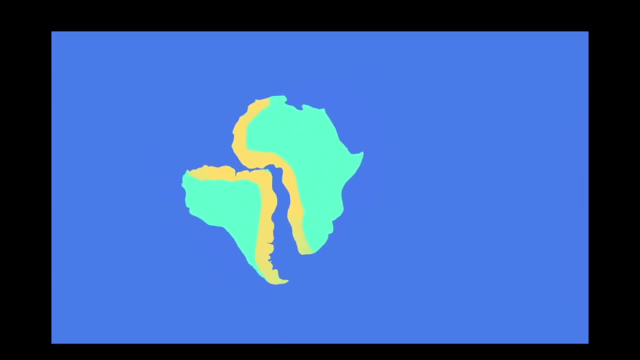 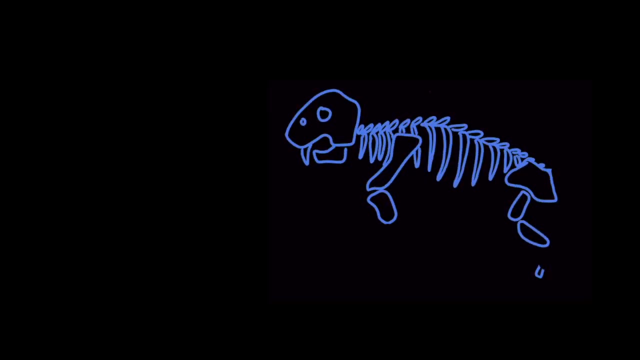 fit into the west coast of Africa. Matching or complementary coastlines is one piece of evidence that continents were once in different locations. Another piece of evidence is that scientists have found fossils from the same species on different continents. There's no way those land organisms 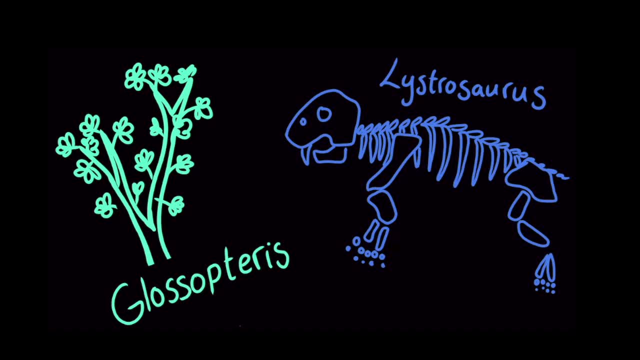 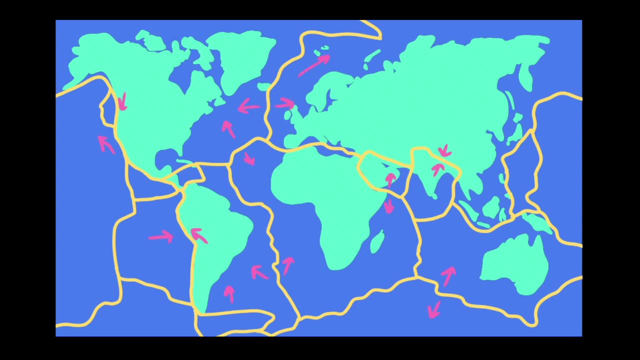 could have traveled across the ocean. This suggests that the animals lived from. the continents were connected And the plates are still moving slowly but surely to this day. But they aren't all moving in the same direction. A plate can collide with one plate, move away from a different. 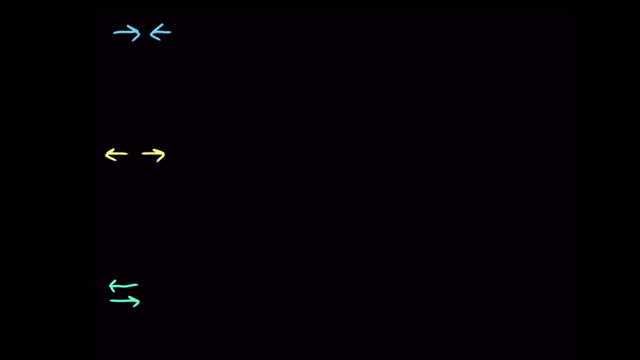 plate and slide past another. We categorize the ways plates interact at their edges as having convergent, divergent or transform boundaries. Con is a Latin prefix, meaning together, so convergent plate boundaries are places where two plates come together. Let's take a look at an 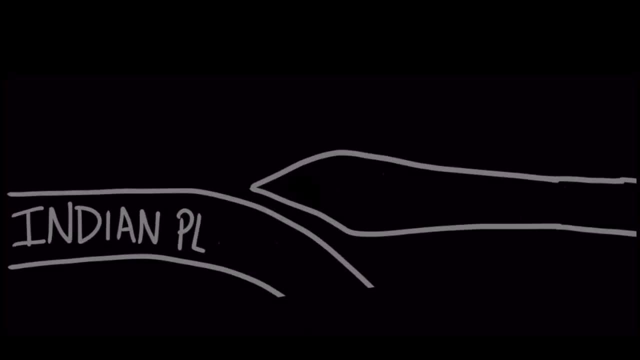 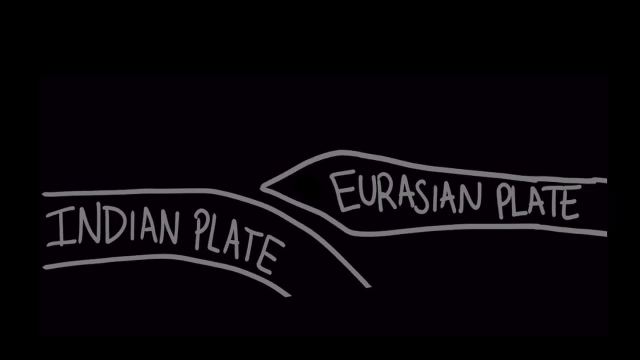 example of a convergent plate. Con is a Latin prefix meaning together, so convergent plate boundary where the Indian tectonic plate collides with the Eurasian plate. The crust of the plate becomes compressed and the Indian tectonic plate gradually moves under the Eurasian plate. 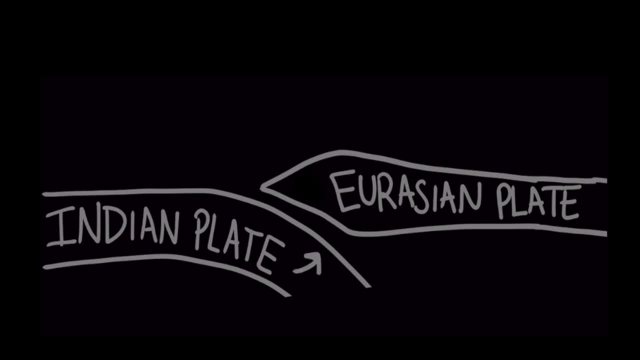 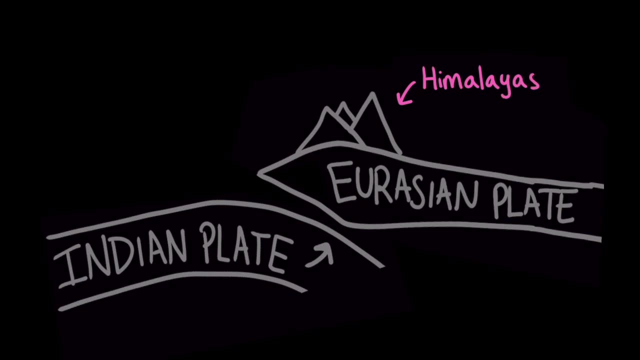 However, the lower density of the crust keeps the Indian plate from sinking back into the asthenosphere all the way. This lifts up the Eurasian plate and creates the Himalayan mountains. These mountains are some of the highest in the world, and they include Mount Everest. 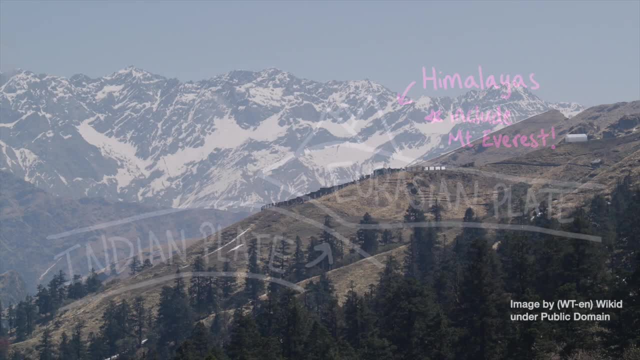 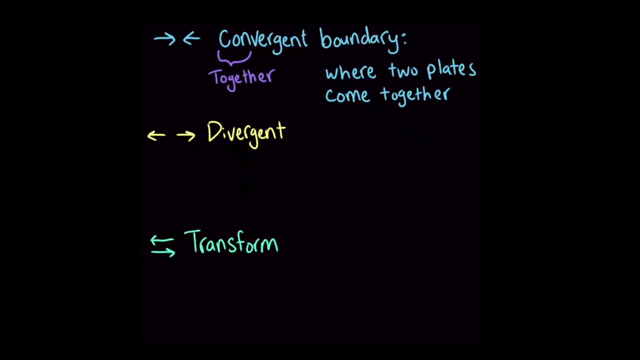 which is the tallest mountain above sea level, And the two plates are still colliding. This causes the Himalayas to grow by more than one centimeter each year. Another kind of plate movement is called a divergent boundary. The di- in divergent comes. 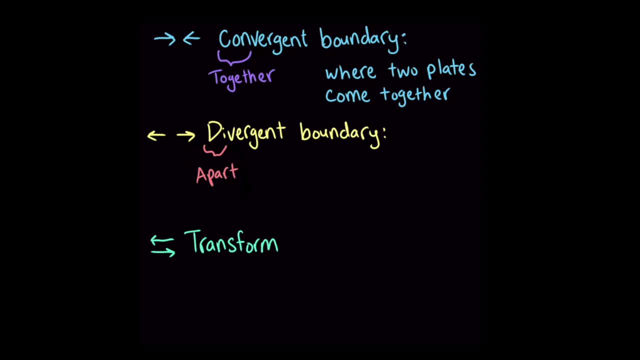 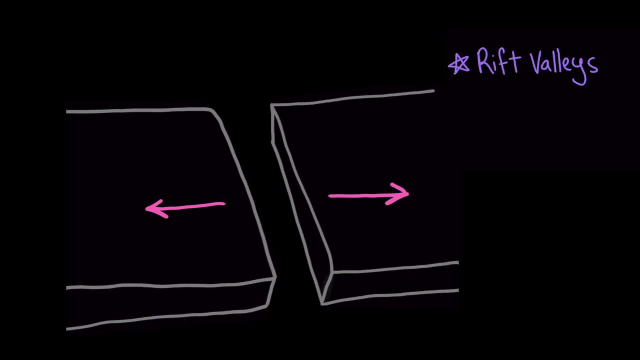 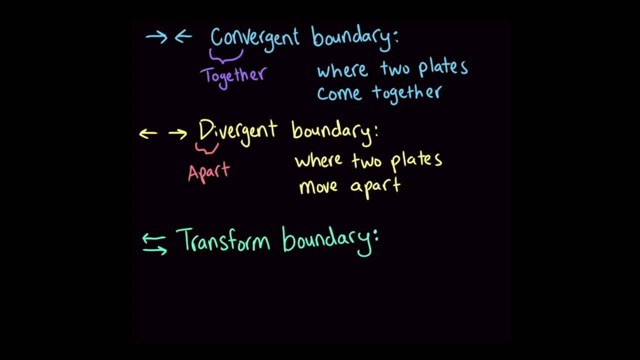 from a Latin prefix meaning apart. so divergent boundaries happen where two tectonic plates move apart. Divergent boundaries can create different kinds of landforms, like rift valleys and mid-ocean ridges. The third kind of plate boundary is called a transform boundary or transform fault, and it 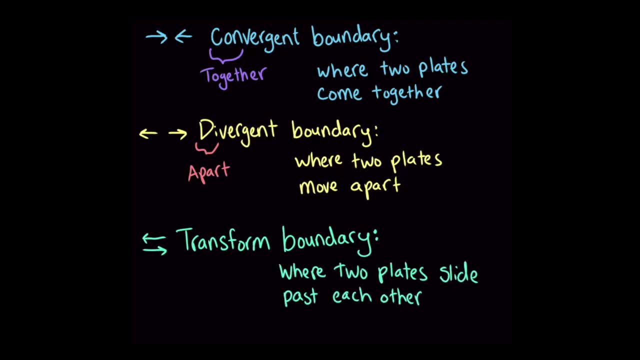 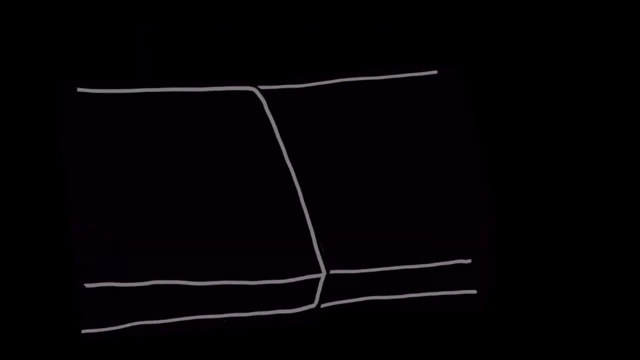 happens when two plates collide with one another. This happens when two plates collide with one another. This happens when two plates slide past each other. Okay, maybe slide isn't the best word for it, because the plates don't move in one continuous motion. You can imagine when two incredibly large, bulky, rocky things move past each other. 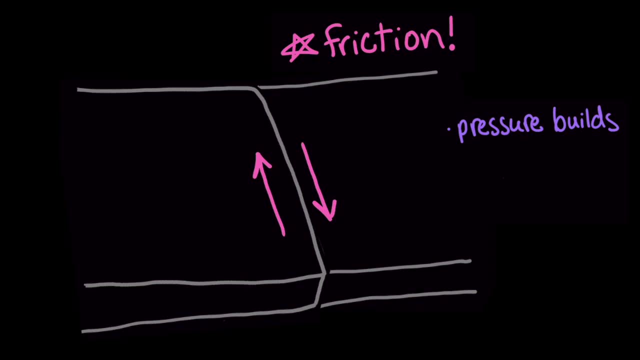 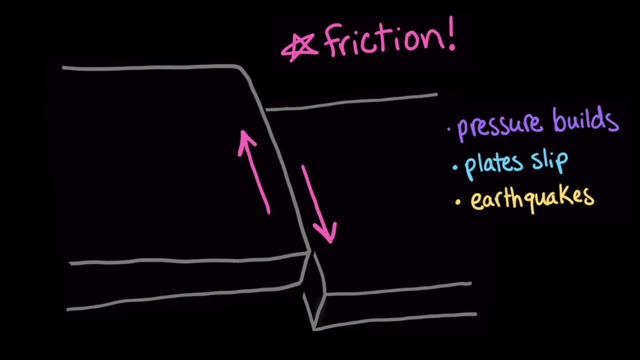 there's a lot of friction, Pressure builds up between the plates and once it gets to be too much, the plates slip and release the pressure. This motion causes earthquakes, And you might be wondering what causes plates to move. Well, scientists are always learning about the earth. 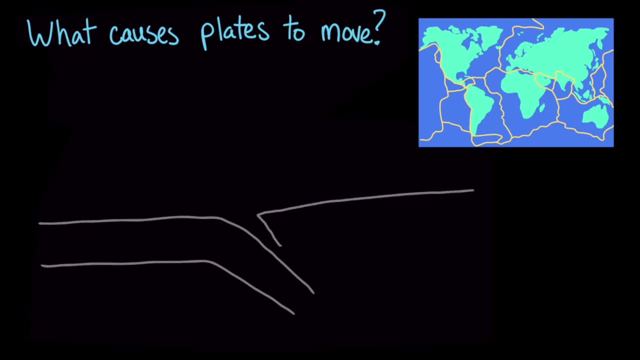 and they're not just about the earth, but about the earth itself. Earth is so complex. Although earth's internal heat may play a small role, more evidence shows that gravity is key. Tectonic plates are solid and they're denser and cooler than the asthenosphere, Because the asthenosphere is also